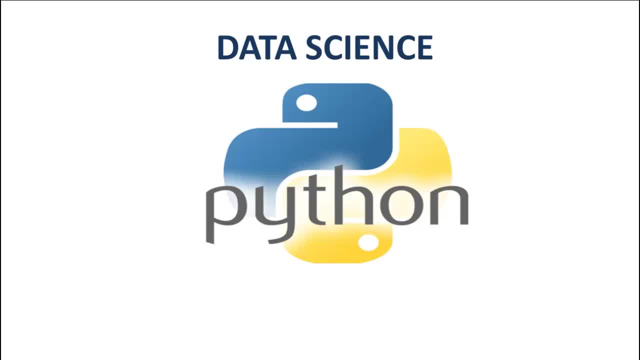 Hello and welcome to another video on python for data science. In the previous video I talked about how the missing values can cause some unexpected results in our analysis and that there is a need to eliminate them. I also showed to use the isNull and the sum functions to count the number of rows that 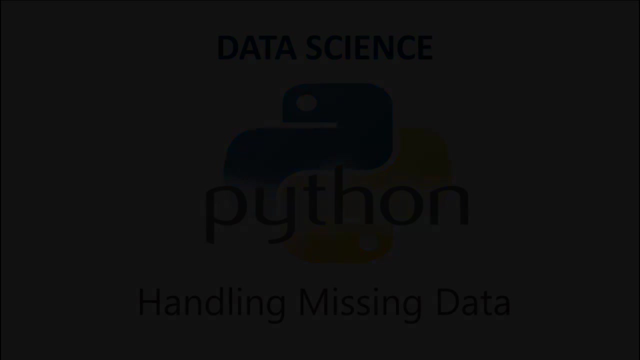 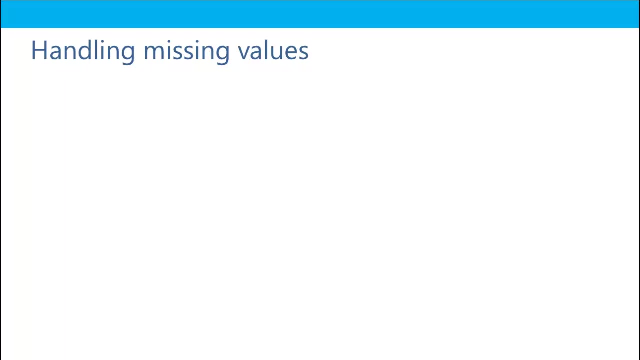 do not contain the missing values. In this video, I will show how we can do analysis on our dataset by removing the missing values. Dropna is a method which drops any row that contains a missing value. However, if all the rows in our dataset contain some one or more missing values, then we may. 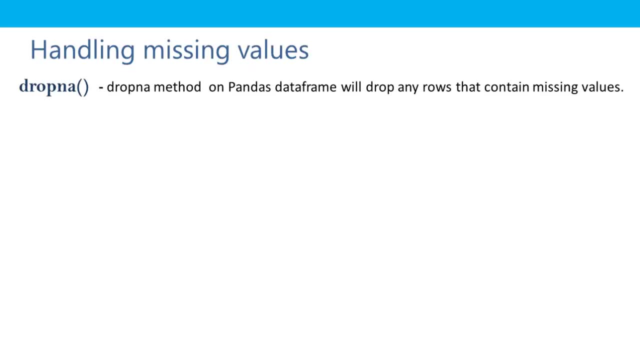 get an empty dataset as our output. So in order to overcome this, we need to use a parameter. This parameter is called subset. The subset will drop the rows of only that column on which we want to do the analysis. For example, if we want to get the mean of the age column, the subset on age column will. 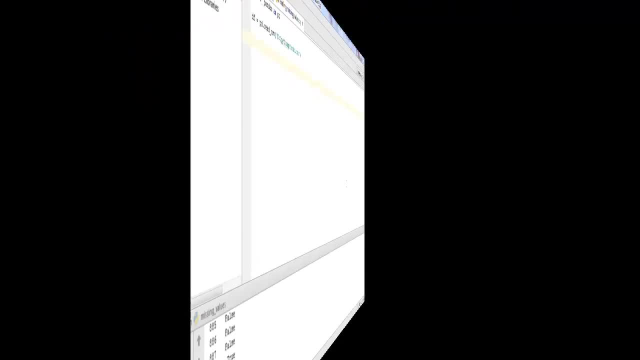 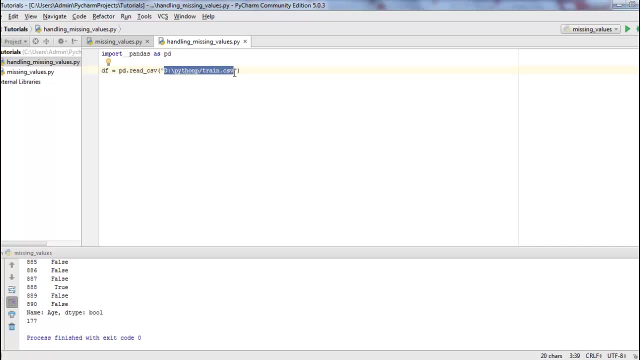 drop all the rows where age is missing. So I have imported pandas as well as read my csv file in a data frame, And I will create a data frame. I will create a simple variable called values And this variable will store all the rows that do not contain the missing values. 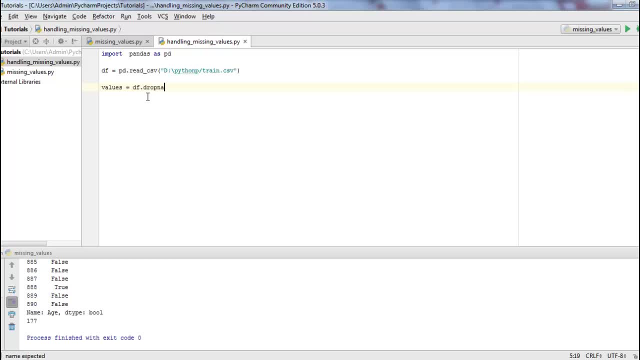 And for that I will be using the dropna method and subset the column age. I will also print valuesshape to see the number of rows that do not contain the missing values. Let's run this and see the result. Okay, So we have 714 rows.